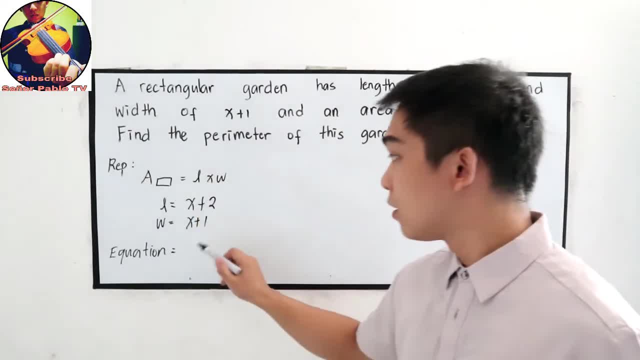 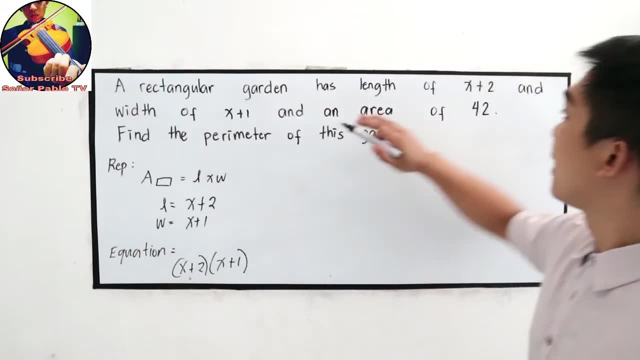 Let us substitute length times the wheel, So length is x plus 2 times the wheel, x plus 1 divided by the width of the garden. So length times the width of the garden. Let's substitute length times the width of the garden, So length is x plus 2 times the wheel, x plus 1. 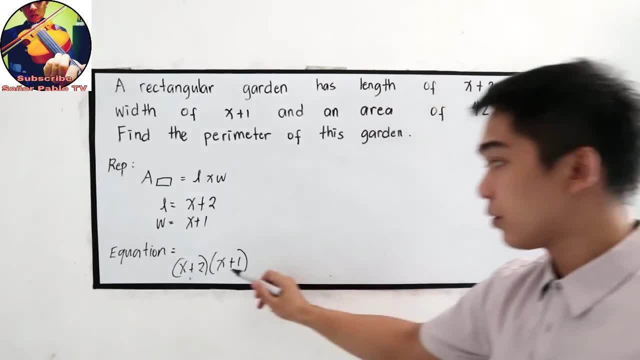 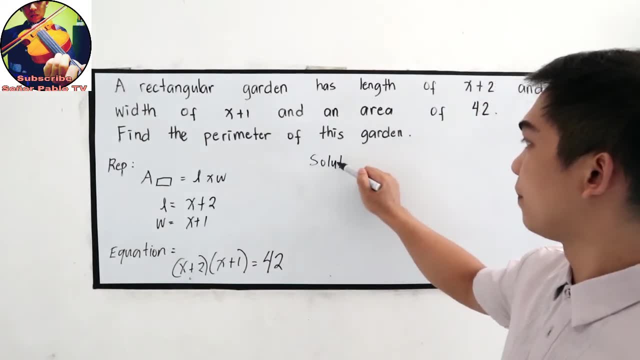 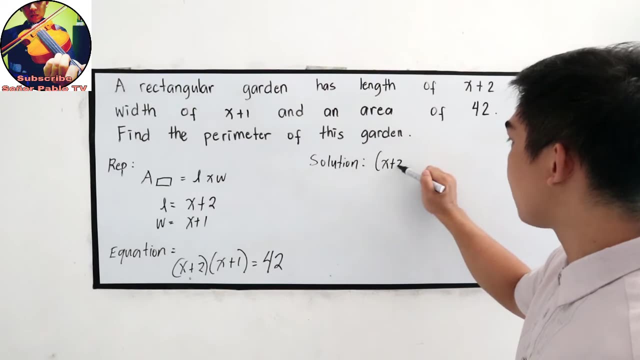 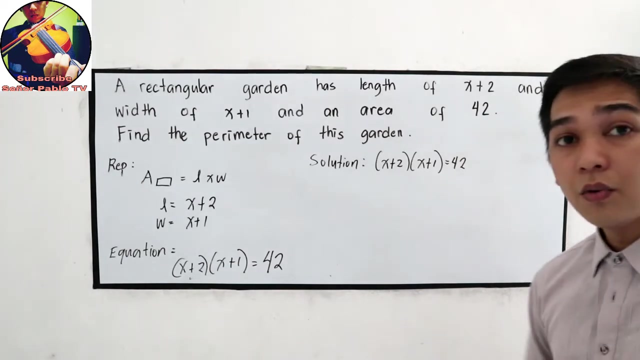 given the area of 42 is equal to 42, let us proceed in our solution. so let us copy our equation: x plus 2 times x plus 1 is equal to 42. okay now foil method: x times x, x squared, x times 1 positive x 2 times x positive 2x. 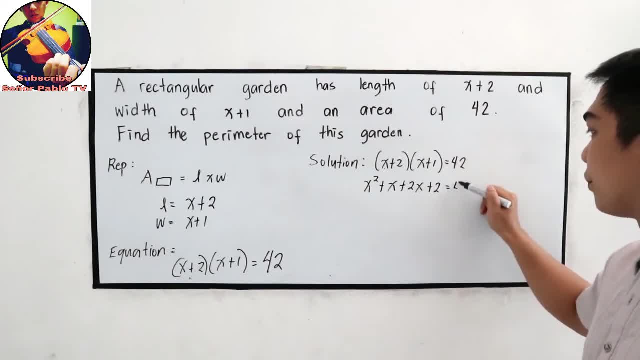 2 times 1 positive 2 and that is equal to 42.. combine like terms so we have x squared plus x plus 2x. that is, 3x plus 2 is equal to 42.. let us transpose 42 on the left side so we have x squared plus 3x plus 2. 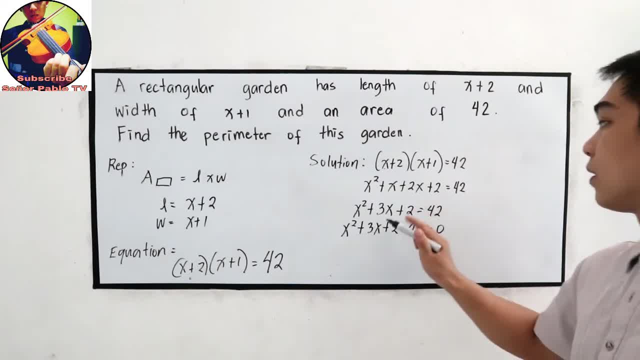 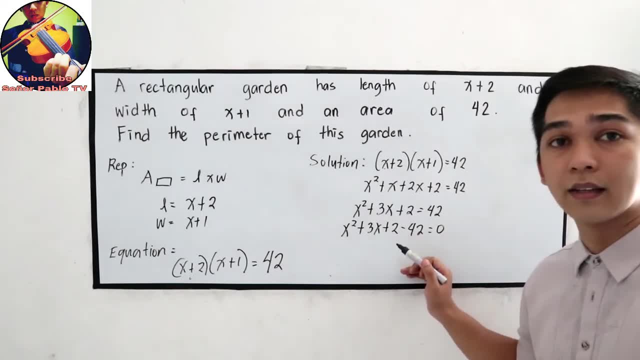 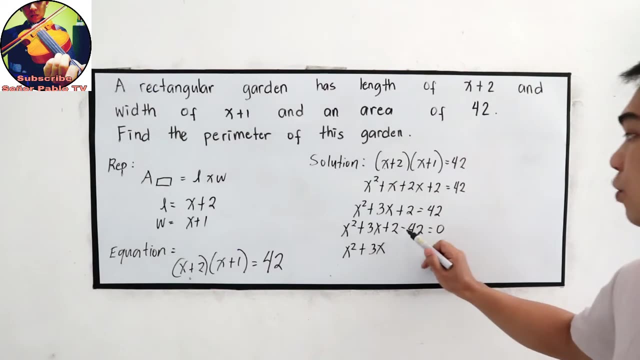 minus 42 is equal to 0.. don't forget: if you're going to transpose one number, you need to change the sign. now let us combine like terms: x squared plus 3x, 2 minus 42 negative 40 is equal to 0.. and now let us find the factors of negative 40.. 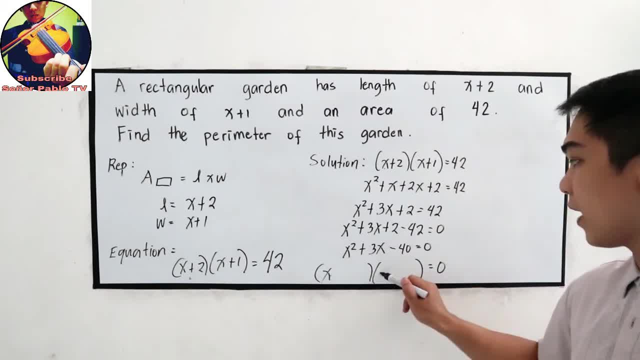 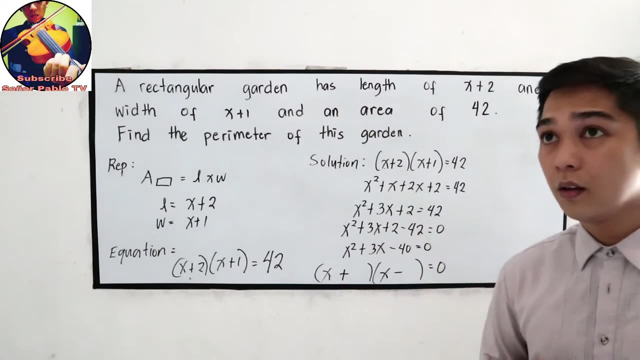 so our factors is equal to 0. so x and x, the factors of x squared, since this is negative. so our factor has a sign of 1 positive and 1 negative, factors of negative: 40. now the sum must be positive because it is a positive. so the quantity of x squared u: 0. emperor and fifty. 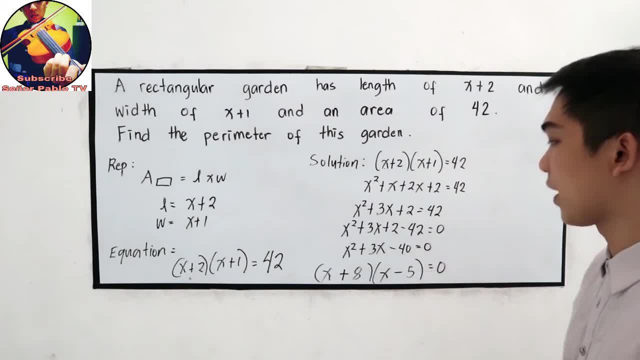 plus a is equal to zero. our time is chili. point two plus two, x plus 3x plus 1, that is x squared plus 2, that is f. neither x squared or y and x squared is the same, so we have x squared plus 8. if you think doubly, you know why five is exactly y. it is because we have x squared as a five or the.